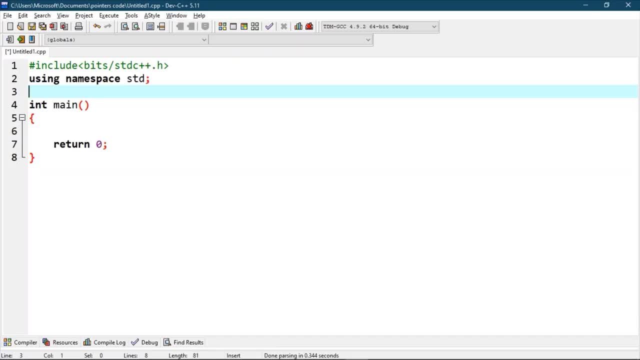 in the code editor. Let's start by creating a node. To create a node, we need a class. Let's declare a class node. Let's create a class node. Let's declare a class node. Let's create a class node. We will declare its member as public. The first member is int. 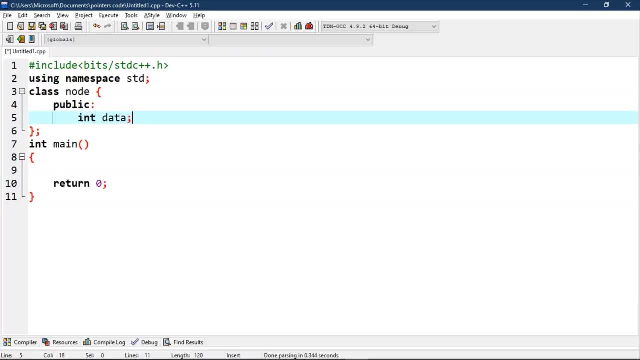 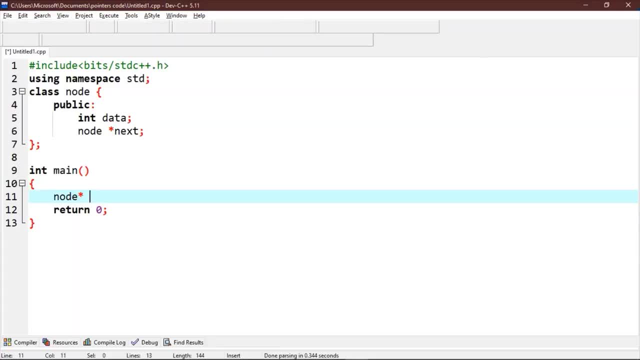 to use node star, The node name had equals to null. Similarly, we will create more nodes To initialize a node. we need to use node pointer next To initialize a node. we need to use node pointer next To initialize a node. we will create more nodes To initialize a new node. we need: 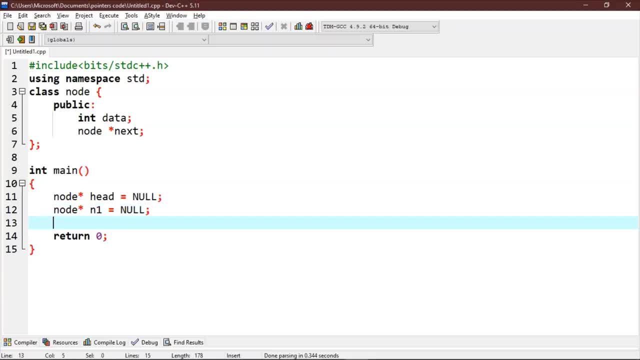 to use node pointer. next, To initialize a new node, we need to have a position called boxside. We will set as of only nonpassive. After that we will set the engine legend to 25.. And here we have our default login for this node. For this icon let's write a kvk password and 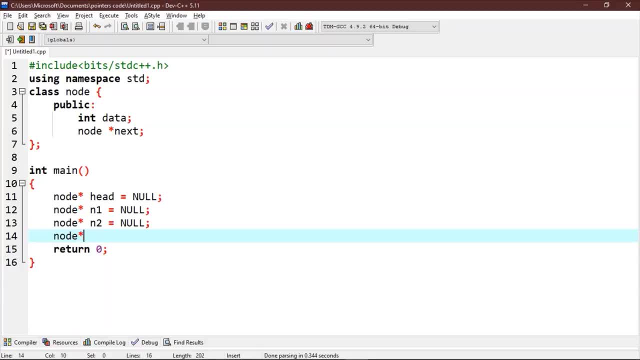 click on this icon to register it. Use this icon to see the result of the newsunit file. Let's click on here Because it is showing us the latest both versions of the 된h Germany. Now we will allocate these 4 nodes in the heap. to do that, we will use a node name equals. 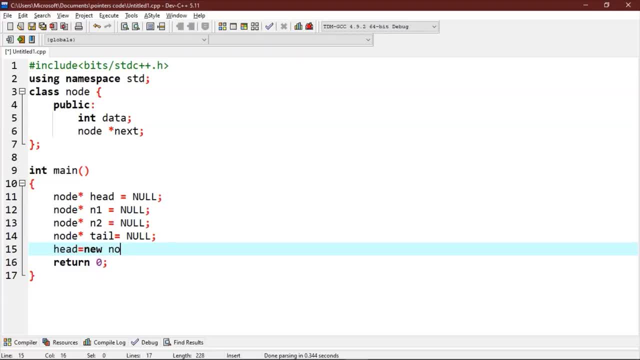 to new node star, new node braces. Now we will allocate all the nodes in the same manner. Now we will assign data to our first node To access the member of the node class. we will use error formation, then we will use data. 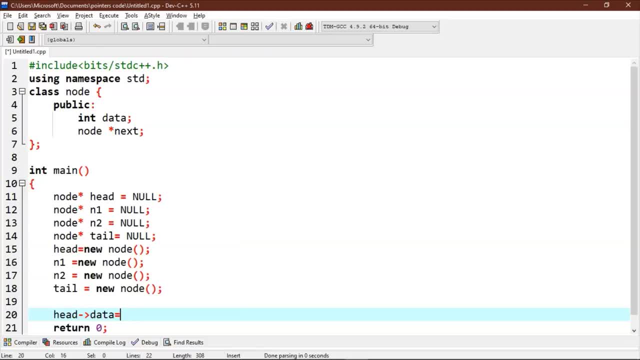 So data equals to: let's give it a value as 2.. Now we will link this first node with our second node. to do that, we will use add, same error formation and next, which will be equals to our n1 node. 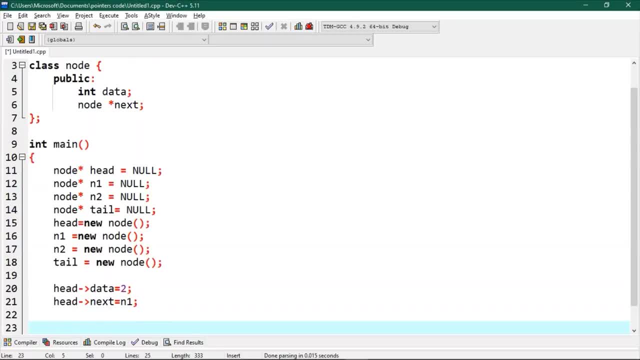 And now we have created a new node. So we have created our first complete node. Now let's create other nodes as well. n1 arrow data is equals to- let's give it 3, n1 arrow next is equals to n2, n2 arrow. 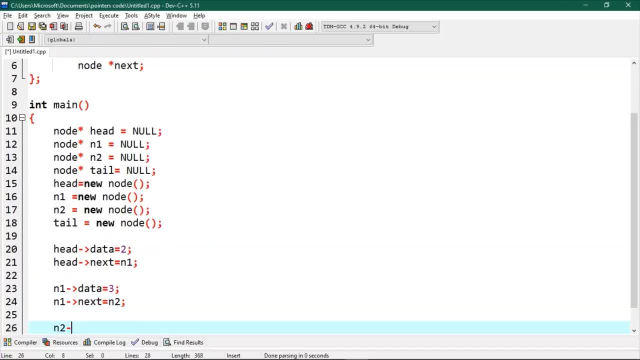 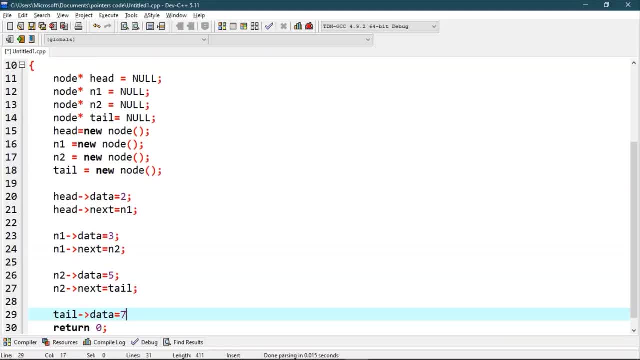 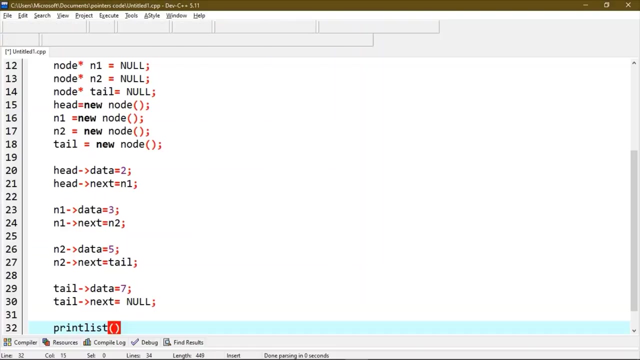 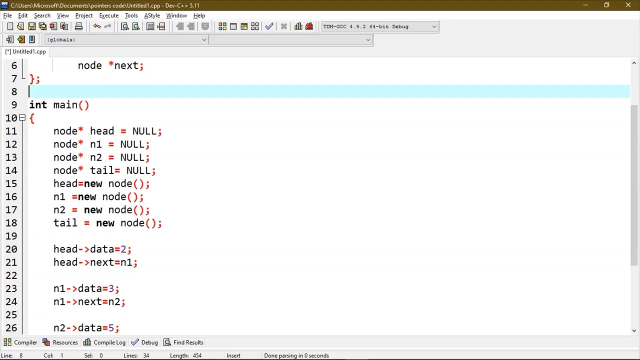 Now let's call a function to print this list. We will give head as the argument. as we can only traverse a linked list from its head, Let's write a definition for this print list function. This function will be a void function. The argument is node star A. We will use while loop to traverse this linked. 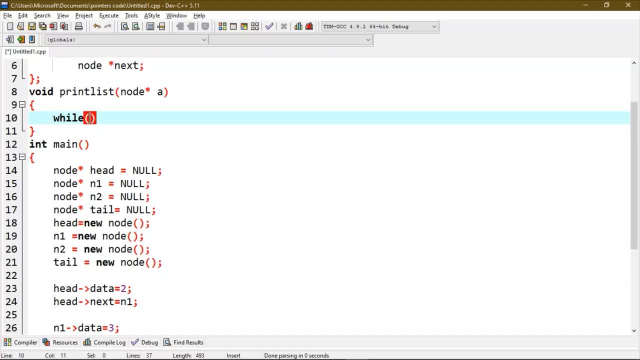 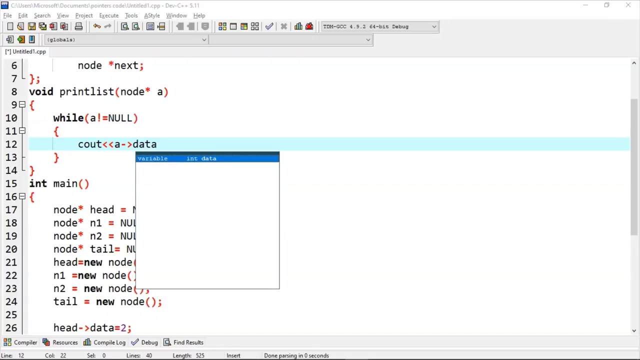 list, We will give its condition. if A is not equals to null, then we will say IN The output is TOUT is A and L. Now we will change our cursor from the current node to the next node to date. To do that, we will use a is equal to a arrow. next, 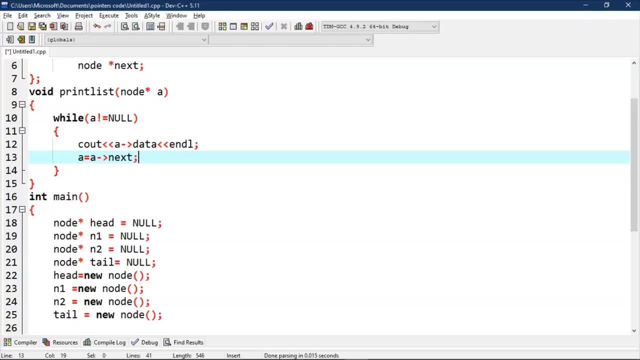 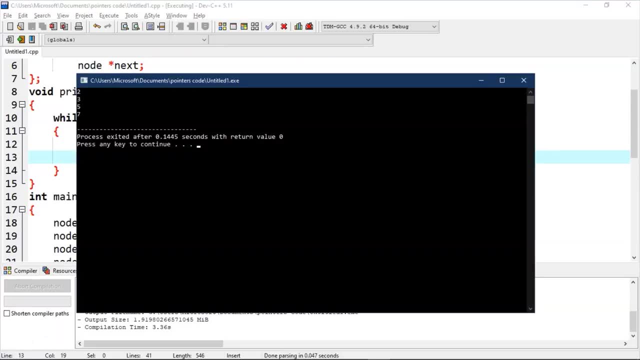 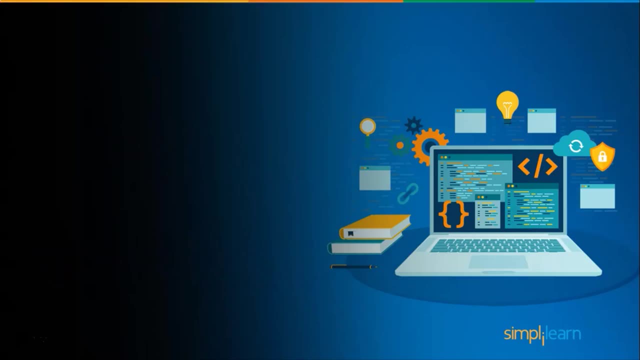 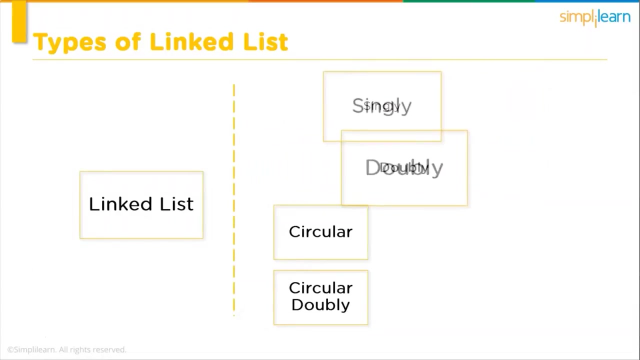 Now let's try to execute this code. As you can see, we have traversed our complete linked list. Now let's get back to our slides. Now let's discuss different types of linked list. The first of singly linked list. next is the doubly linked list, the circular linked list. 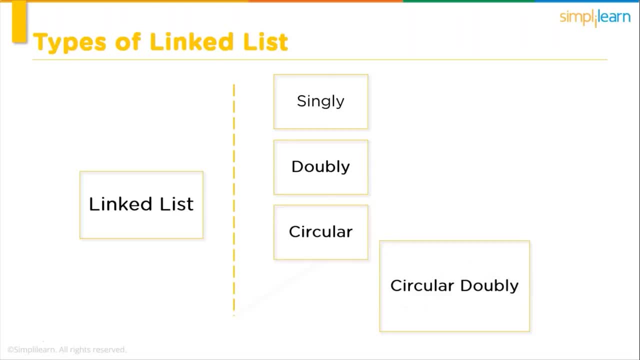 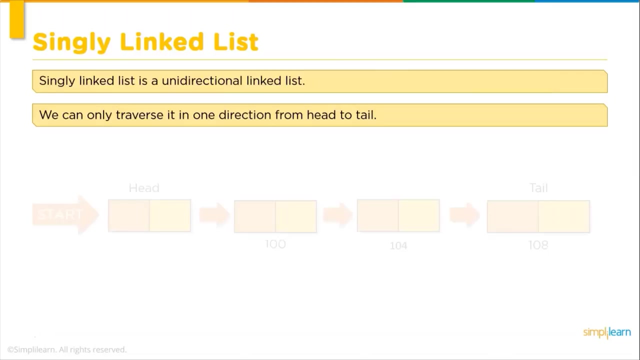 and finally, we have the circular doubly linked list. Let's discuss each one of these in details. First up, singly linked list. It is a unidirectional linked list. While using the singly linked list, we can only traverse it in one direction, that is. 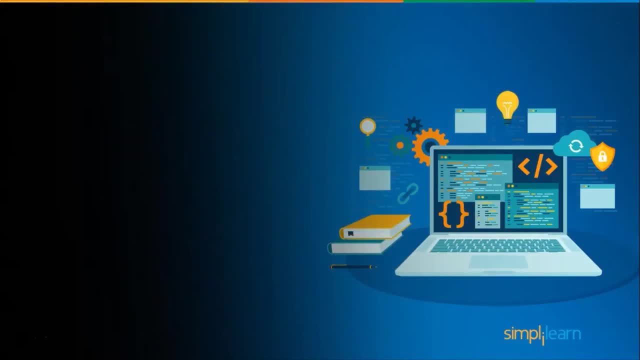 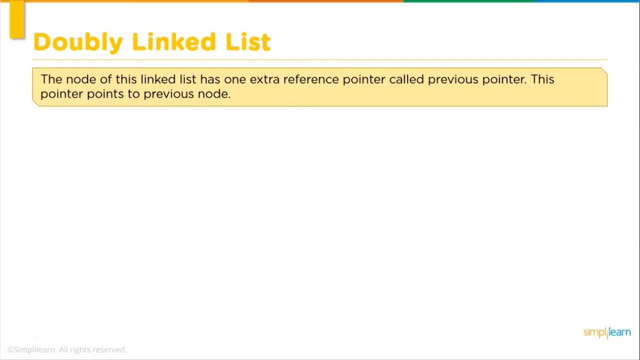 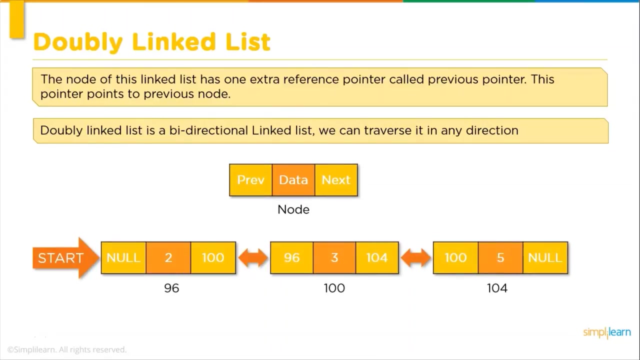 from head node to the tail node Next up doubly linked list. It is a bidirectional linked list. we can traverse it in both the directions. In this linked list the node has an additional pointer that points to the previous node. Next up, circular linked list. 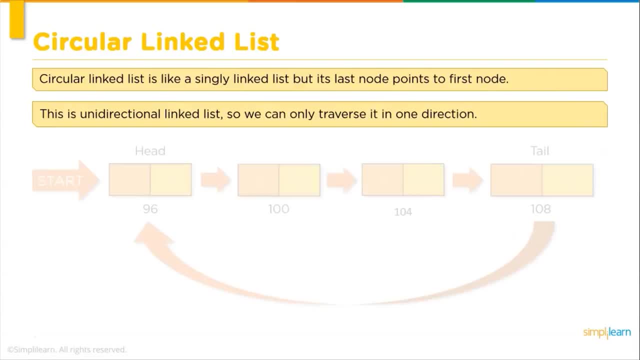 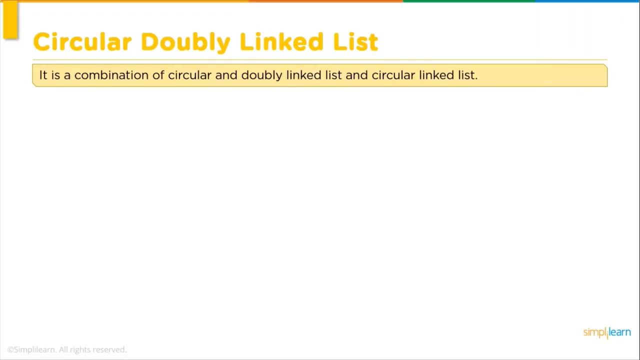 It is a regular linked list, except for its last node points to the head node. Programmer needs to be careful while traversing it or they might get stuck in an infinite loop. Next up, the circular doubly linked list. It is a combination of doubly linked list and a circular linked list. 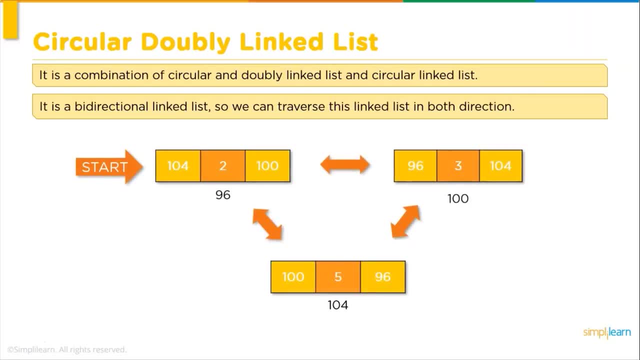 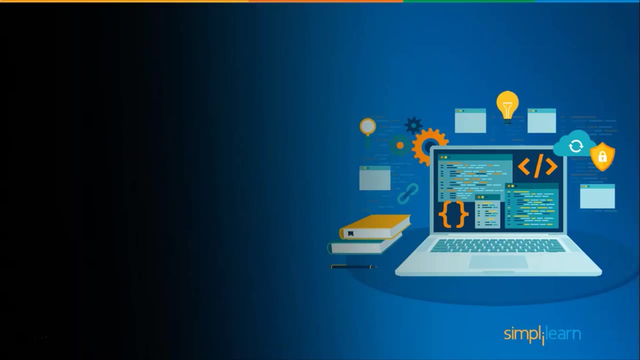 Its last node points at the head node and the previous pointer of the head node points to the last node. It is also bidirectional linked list so that we can traverse it in both directions. We have now discussed the linked list. why do we need linked list and types of linked. 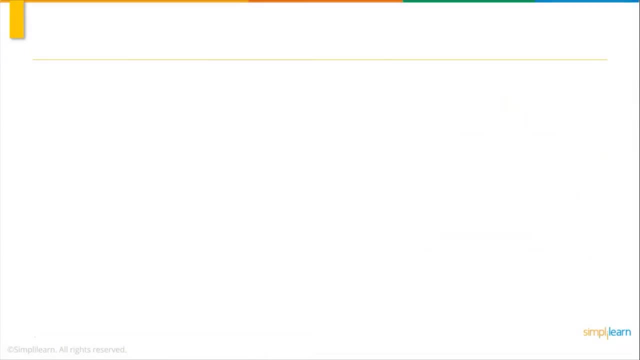 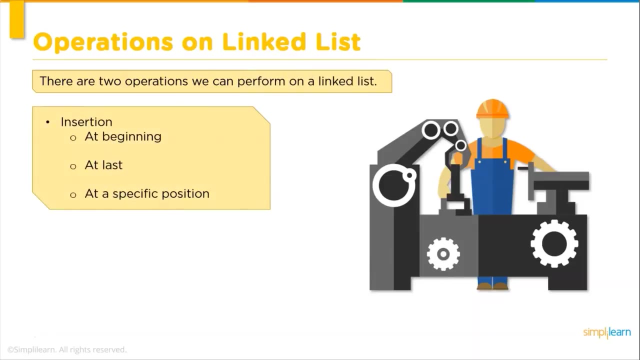 list. Now let's learn about some operations we can apply on linked list. We can use majorly two operations on linked list. First up, insertion and deletion. We can perform these operations in three different situations. first, at the beginning, at the 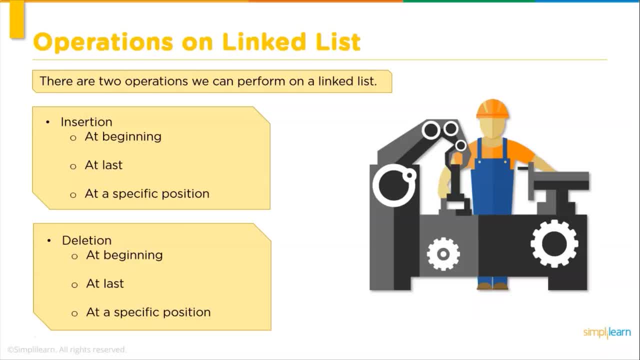 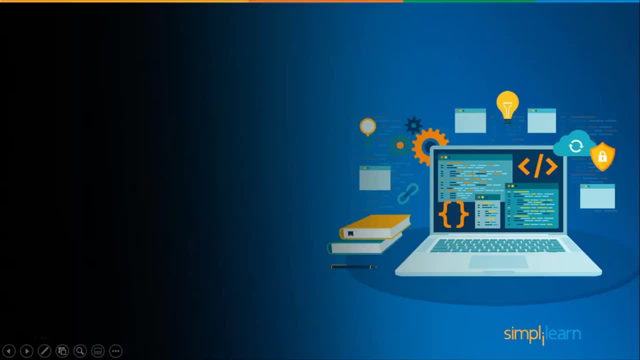 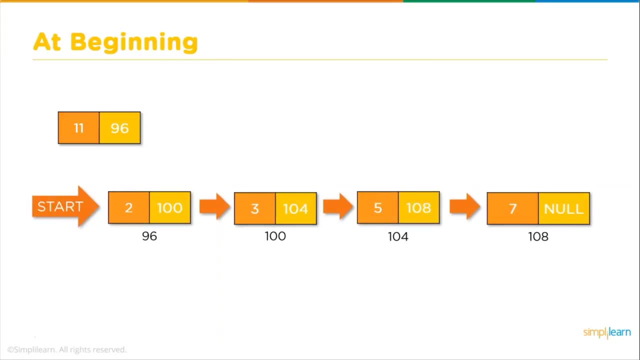 last or at a specific position after a node. Next we will discuss these operations in detail. Let's start. 1. First up, insertion. We will discuss first insertion. at the beginning We have to give the first node's address to the new node's next pointer, to execute. 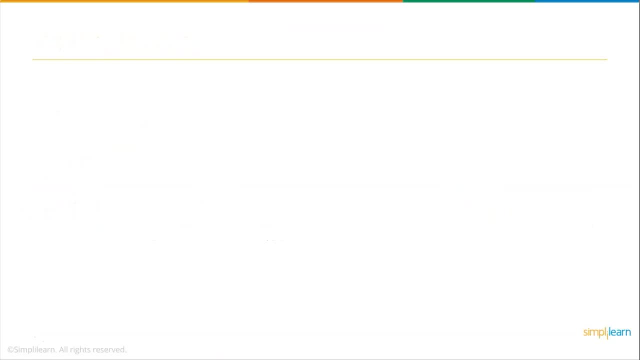 this Next up insertion at the end We have to give the new node's address to the last node's reference pointer. Next up insertion at a specific position. To do this we will have to change the reference address of the previous node to the new node's. 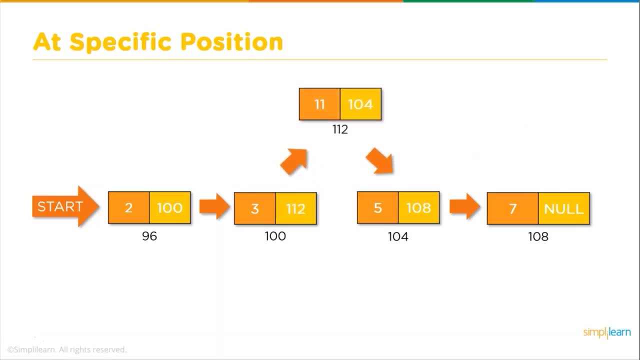 address and the new node's reference pointer to the next node's address. Now let's discuss deletion 1.. First up deletion: at the beginning We have to change the first node's address to the null to execute this 2.. 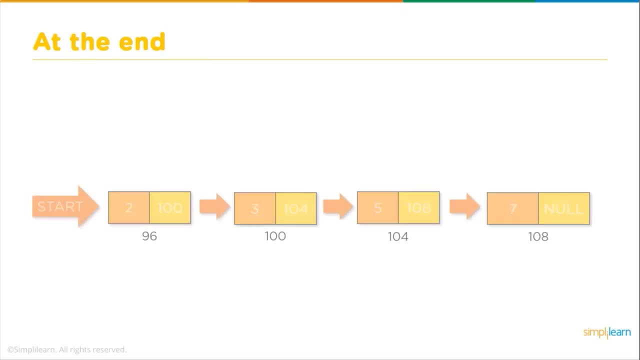 Next up deletion at the end. 3. Next up deletion at the end. We have to change the second last node's address to the null Next up deletion. at a specific position, We will change the reference address of the previous node to the next node's address. 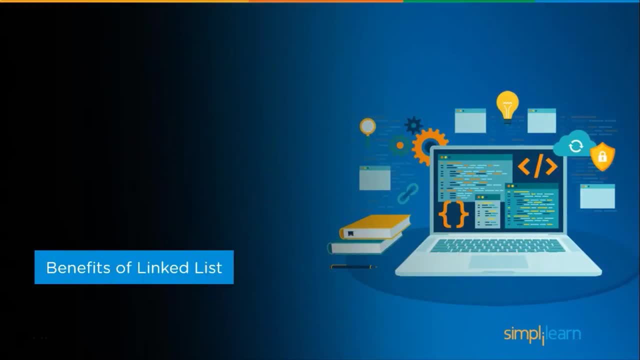 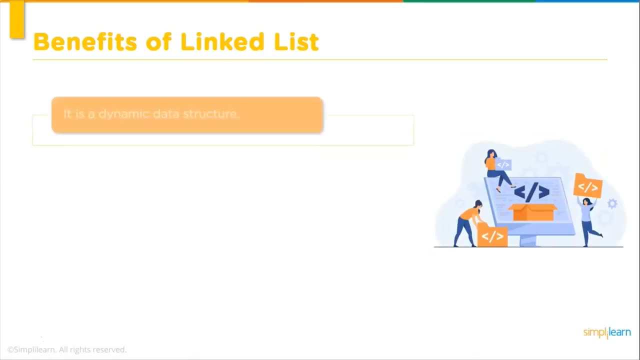 We have learnt a lot about linked list during this session. Now let's discuss some benefits of linked list. 1. First up, Dynamic data structure, ie we can dynamically increase its size. 2. It offers easy insertion and deletion than other linear data structures like arrays and 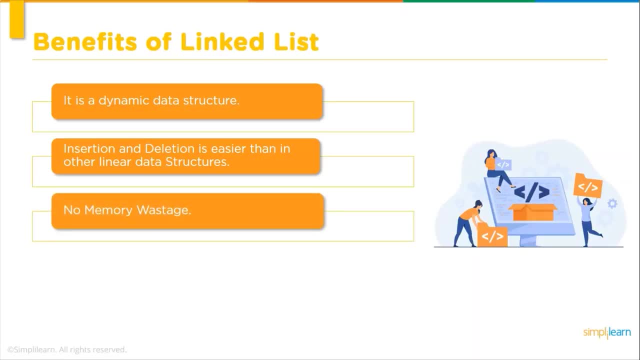 string. 3. Since it can dynamically increase its size, resulting in no memory wastage. 4. It is pretty handy in implementing complex data structures like stacks and queues, etc. Now let's talk about some disadvantages as well. 1. First up. 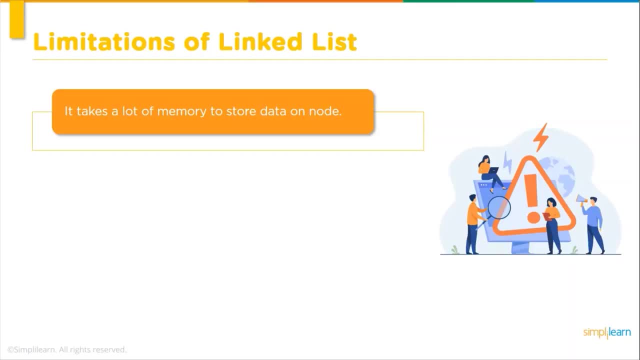 Since the linked list is made up of nodes, it takes extra storage for storing data and reference pointer 2.. Next, the traversal in the linked list is a bit harder than other data structures. 3. Reverse traversing is easy in doubly and circular doubly linked list. 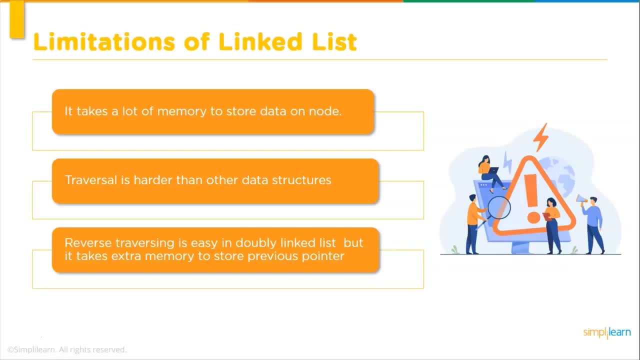 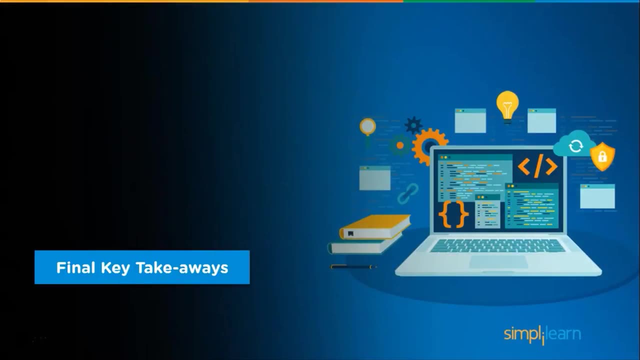 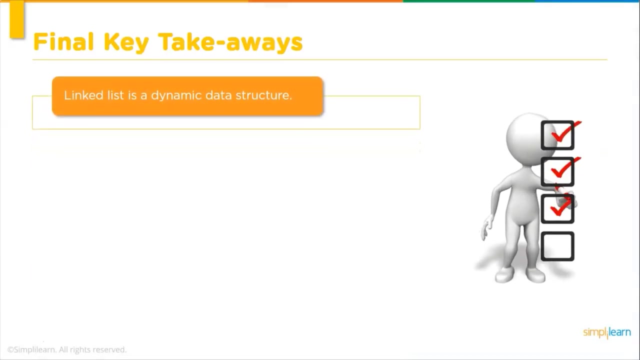 4. Since it uses one extra pointer, it takes extra storage, making it another limitation. At last, let's sum up what we have learnt in this session with key takeaways. 1. First up, we have recognized linked list as a dynamic data structure. 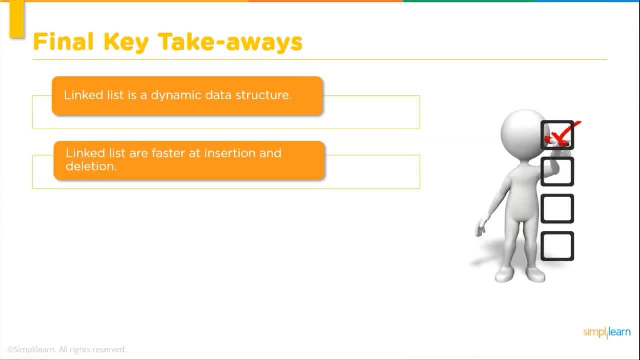 2. Next, a linked list offers faster insertion and deletion operation. 3. Next, linked list: traversal is hard. 4. We have to start from the head node every time. 5. Finally, a linked list is an asset in implementing other data structures like stacks and queues. 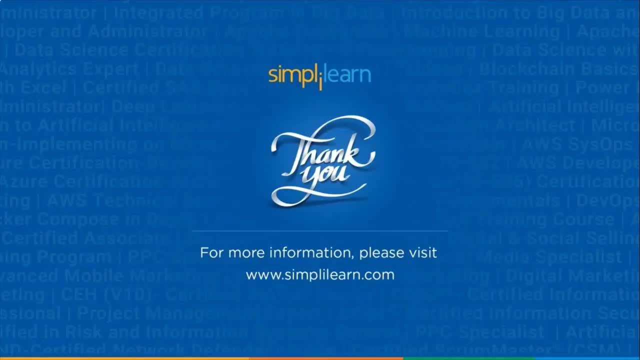 And this was all for today's session. Hope you guys found it informative and helpful. If you liked this session, then like share and subscribe. If you have any questions, then you can drop them in the comment section below. Thanks for watching and stay tuned for more from SimpliLog.